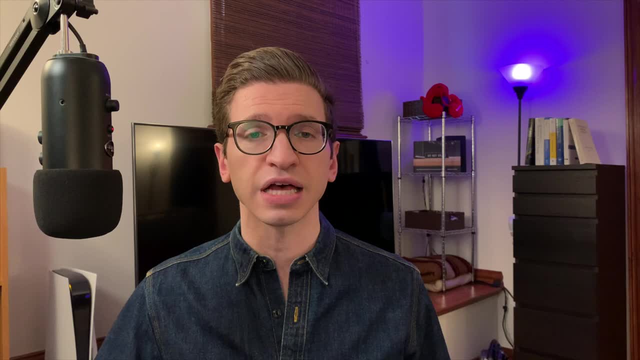 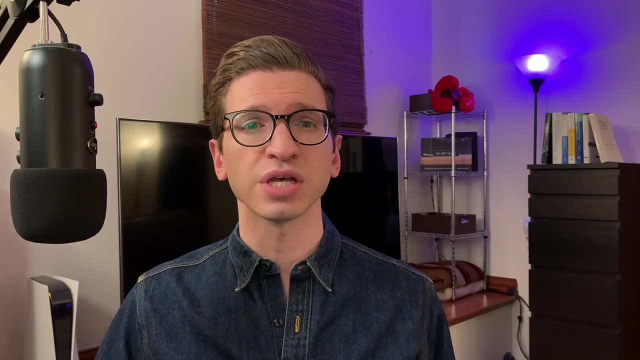 that underlies a huge amount of what we humans have learned about the world in the last few hundred years, from Newtonian mechanics to relativity, to quantum mechanics and quantum field theory. The basic idea goes like this: Say we have a particle that's traveling from point A to point B. What path is it going? 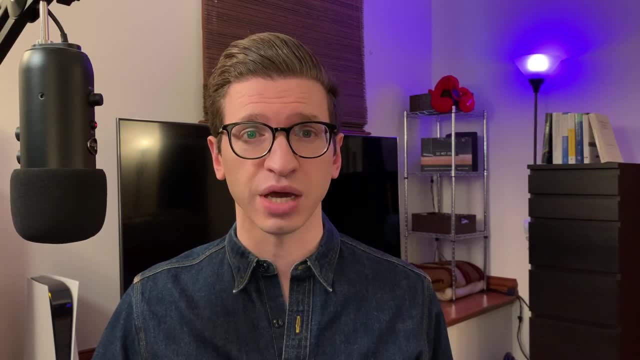 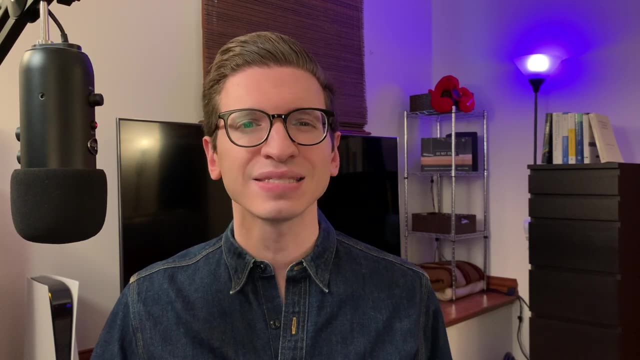 to follow to get there? Newton gave us one way of answering that question, But in the 17 and 1800s Lagrange and Hamilton and others came up with a different proposal. They assigned a number to each possible path, called the action. 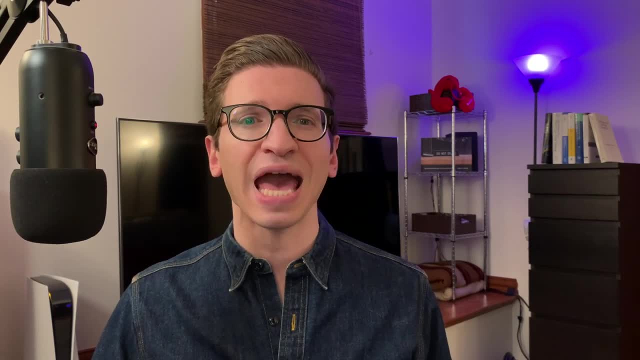 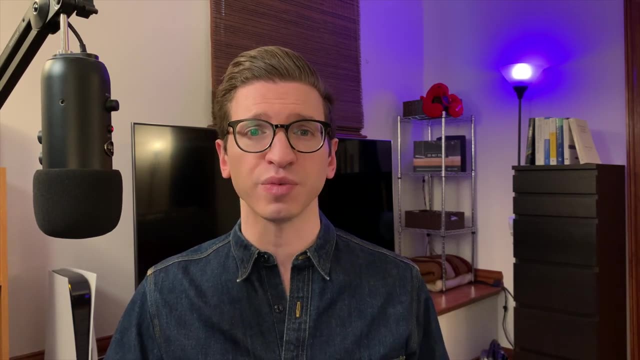 And they showed that the trajectory the particle follows is the one for which the action is minimized. Actually, in quantum mechanics, Feynman showed that the particle in a sense traverses all the possible paths between point A and point B, and the path of least action is the one. 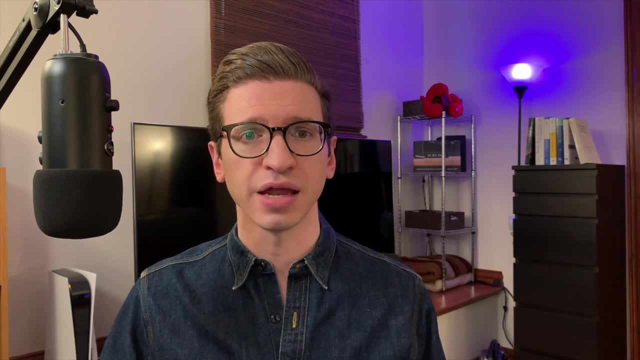 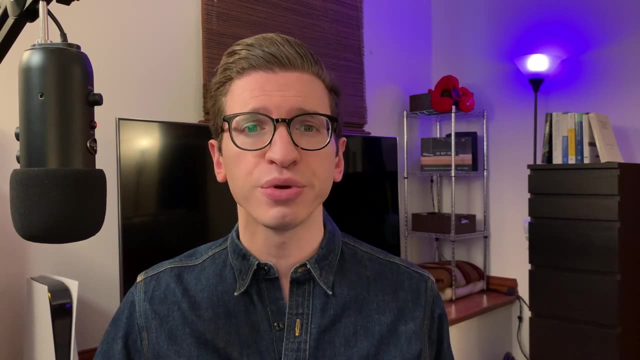 that dominates classically. I'll tell you a little bit more about that, But I'm getting ahead of myself. In this video, I'm going to explain the principle of least action and show you how it reproduces the equations that you already know and love from Newton's laws. 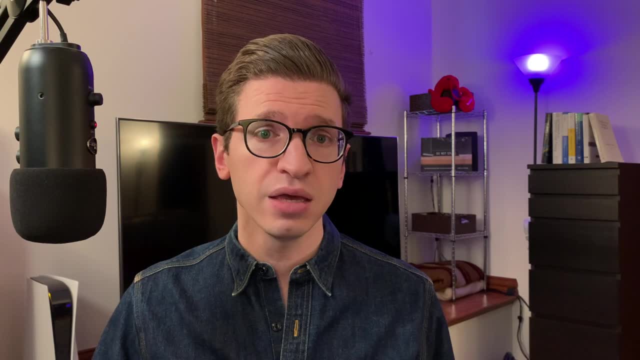 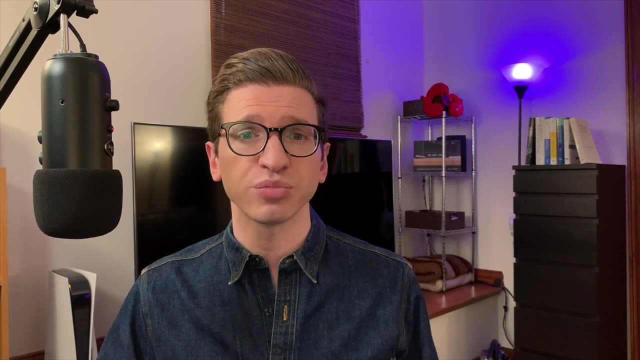 As far as prerequisites go, I'll just assume that you're familiar with F equals ma with potential energy and some basic calculus. This is the first in a series of videos that I'm working on in which I hope to show you the action principle not only in Newtonian mechanics, but in special relativity and 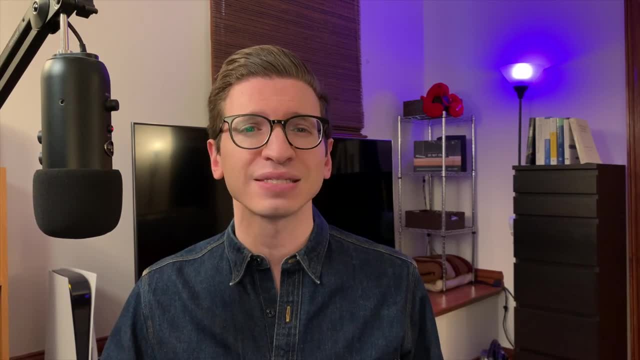 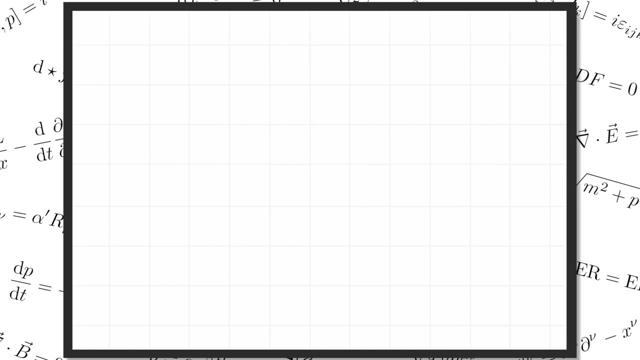 general relativity and even in string theory too, All in as accessible a way as possible. So make sure you're subscribed to the channel if you want to learn all about that and let's get into it. So again, the basic question that we want to answer is say we have a particle of mass. 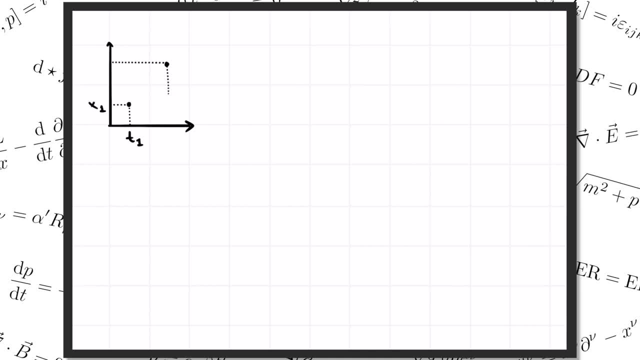 m that travels from point x1 at time t1, to x2 at time t2.. Then what trajectory x of t is it going to follow to get there? I'm going to work with one spatial dimension x here in order to keep things from getting. 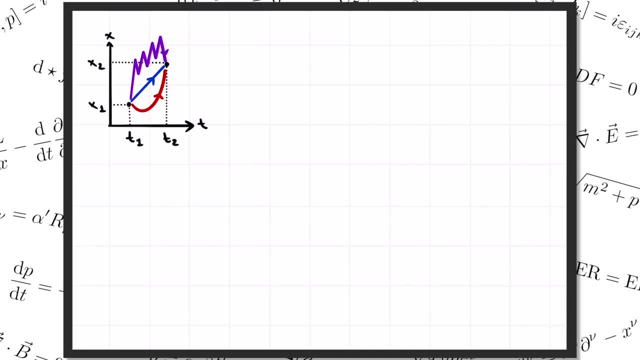 unnecessarily complicated. But of course all of this discussion will generally take a little longer. Newton told us that to answer this question we should write down all the forces on the particle, add them up and then set that equal to the mass times, the acceleration. 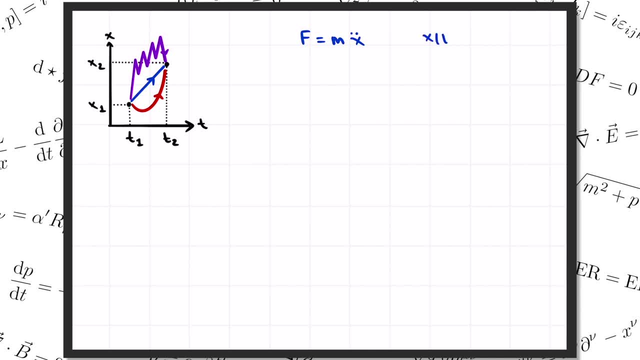 F equals m times x double dot. X of t here stands for the trajectory of the particle. That's what we'd like to solve for here. The dots denote rates of change. So x dot is the velocity function and x double dot is the acceleration function. 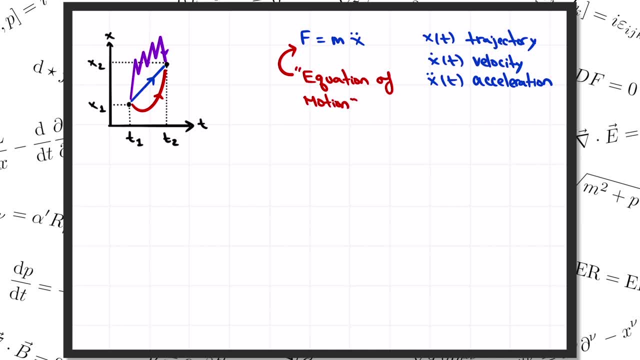 This equation is called the equation of motion. So if you want to solve the equation of motion, you just have to write down all the forces on the particle, add them up and then set that equal to the mass times the acceleration. It's a second-order differential equation that we would then need to solve to figure. 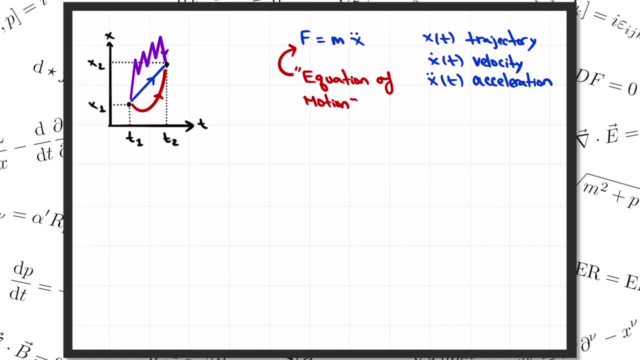 out x of t, But that's a math problem. The physics is about how we write down this differential equation in the first place, And Newton gave us one way to do it. This video is going to be about finding another way to get at these equations. 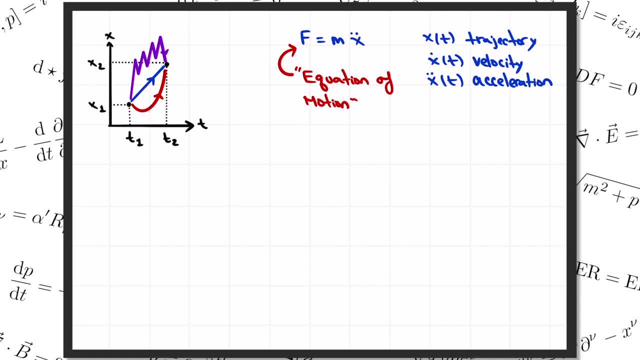 You may have learned before about how the force f is related to the potential energy function u. If not, I made a video about it that I'll link up in the corner. The relation is that the force f is related to the potential energy function u. 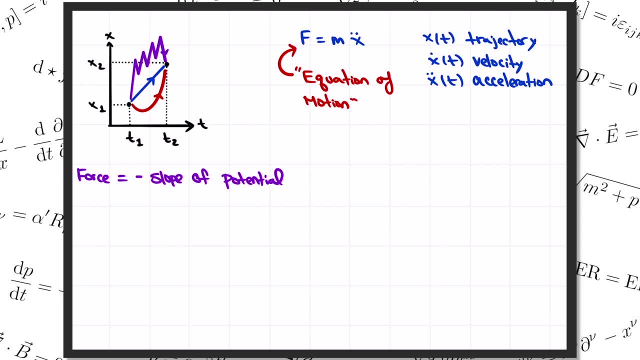 The relation is that the force f is related to the potential energy function u. The strength of f is related to f. of x, The mass is related to the mass of x. The potential energy of x is minus the slope of the potential energy curve. 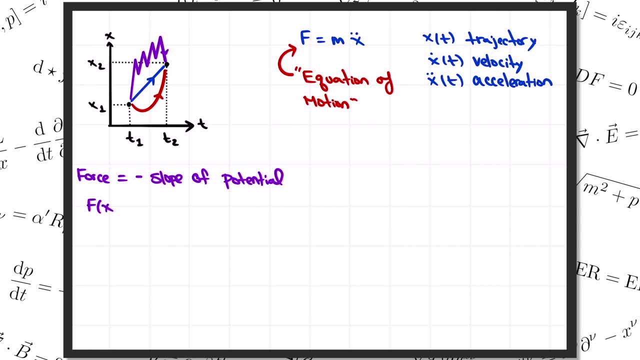 And in an equation that means that f of x is equal to minus the derivative of u with respect to x. To give a couple of examples, for gravity acting on a projectile, the potential is: u equals mg x or mg y, if you prefer to label the height, y. 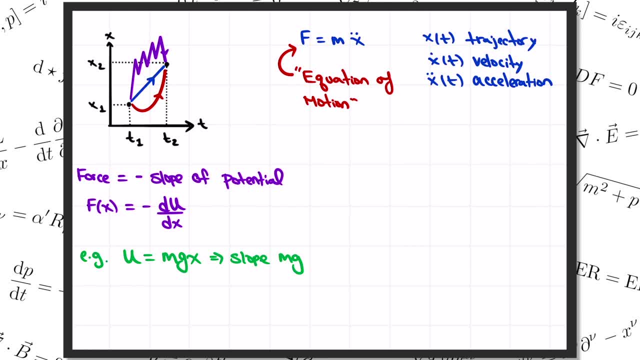 That's just a straight line with slope mg, And so the force is minus that minus mg. Or for a mass on a spur spring, the potential energy is: u equals one half kx. squared. The slope of that is just k times x, and so we get the spring force: f equals minus kx. 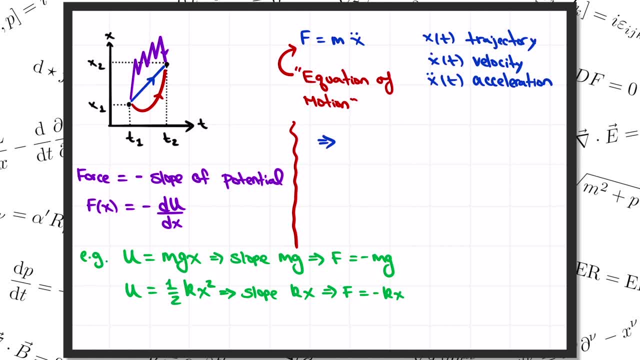 So, in terms of the potential energy, we can rewrite our equation of motion as: mx double dot equals minus the derivative of u with respect to x. Now I want to show you the new root to this equation. Just like we can write down the potential energy u, we can also, of course, write down the kinetic energy k. It's one. 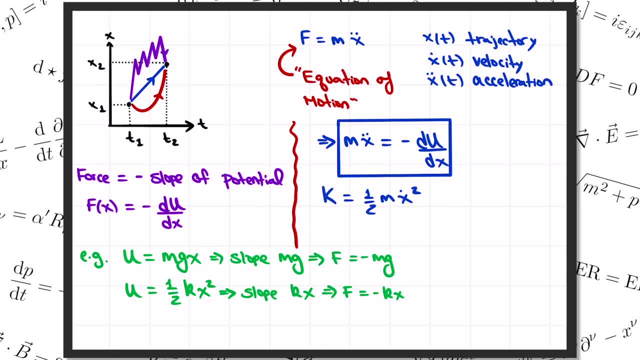 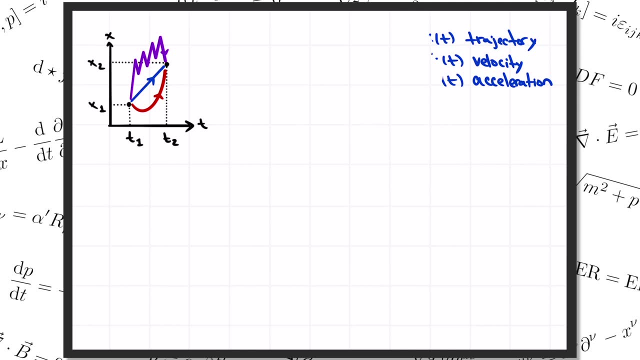 half m times x dot squared, where again x dot stands for the speed of the particle. Their sum e equals k plus u is of course the total energy, But actually right now we are going to work with the difference k minus u. 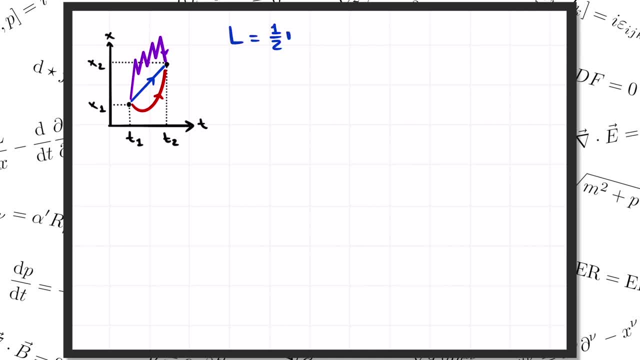 So let's define a function by taking one half m x dot squared minus the potential u. So let's define a function by taking one half m x dot squared minus the potential u. This combination is called the Lagrangian L, And right now it might look like it's coming. 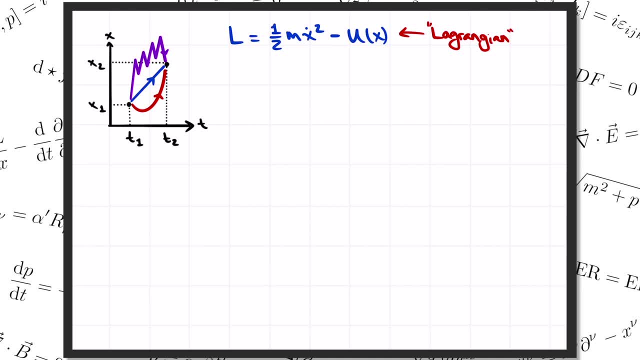 out of left field, but let's see where it leads us. For any path x of t between the particle's starting position and its ending position, we can define a number s by integrating the Lagrangian along the trajectory. So that's the integral from the starting time, t1, to the final time, t2, of one half m x dot. 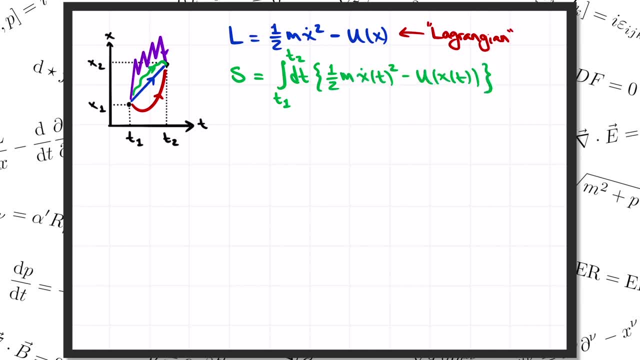 squared minus u. This quantity is called the action And again it's a number that we can assign to any curve, And so far, x of t can be any curve connecting the two given endpoints. Our goal is to use the action to figure out the actual trajectory that the particle is. 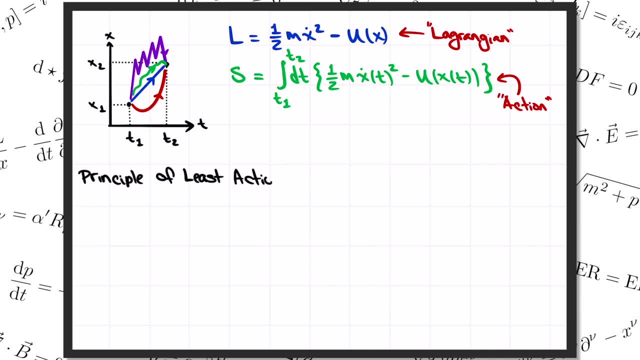 going to follow. And here's the claim. The particle follows the trajectory that minimizes the action, And obviously that's why this is called the principle of least action. Actually, minimized is a little bit too strong of a word here. There can be situations where the solution is a saddle instead of a minimum. 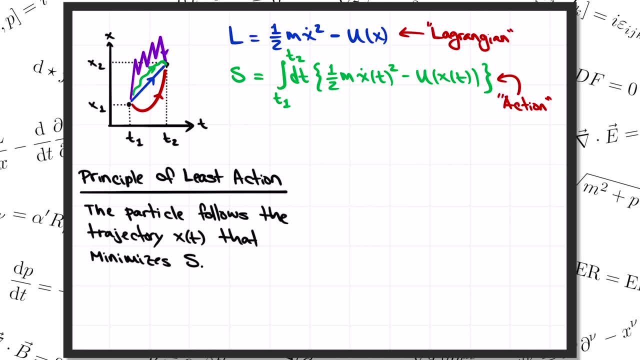 But let's focus on the typical case where s is minimized. So how do we see that this claim is true? Well, think back to your calculus classes, where you had some function f of x and you were asked to find its minima, maxima or saddle points. 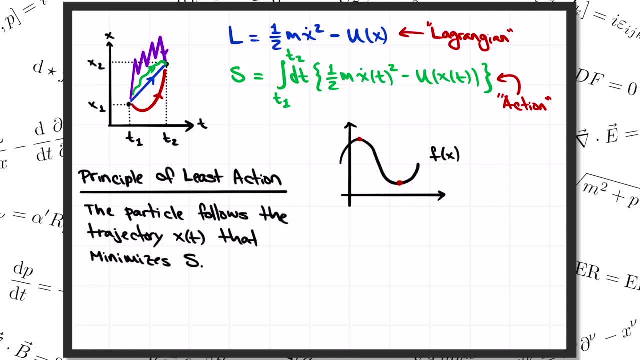 These are called extremal or critical points. They're the points where the slope of the function vanishes. So f prime of x is equal to zero. To say that another way, let's look at the function at a tiny distance, epsilon away from. 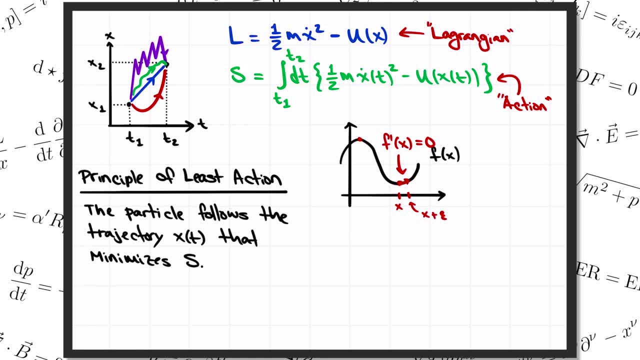 the minimum x. We can tailor expand around x just like any function. So f of x plus a tiny number, epsilon is equal to f of x, the leading term when epsilon is equal to zero, plus the first correction, which is f, prime of x times the displacement. 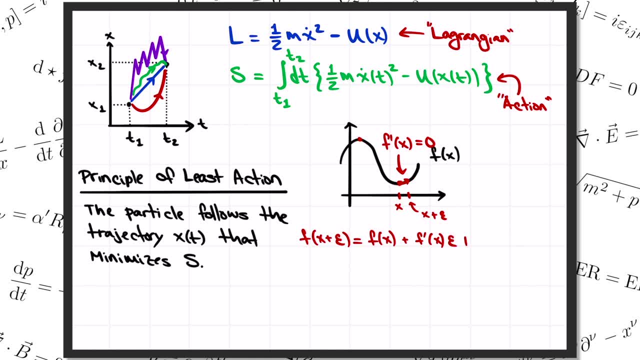 epsilon. And then we have the higher order corrections, Like one half f, double prime, Epsilon squared. But if x is a minimum, then because f prime of x equals zero, the leading term in epsilon vanishes. In other words, when you take a little step, epsilon away from an extremum to leading. 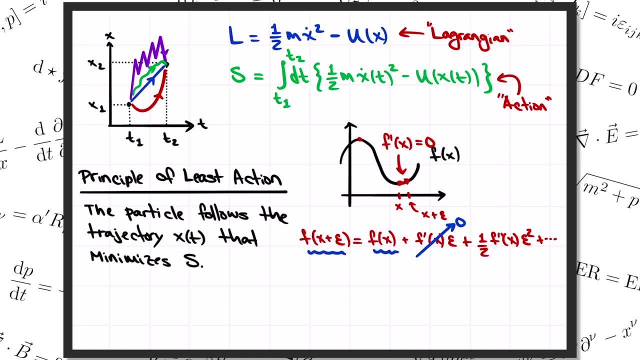 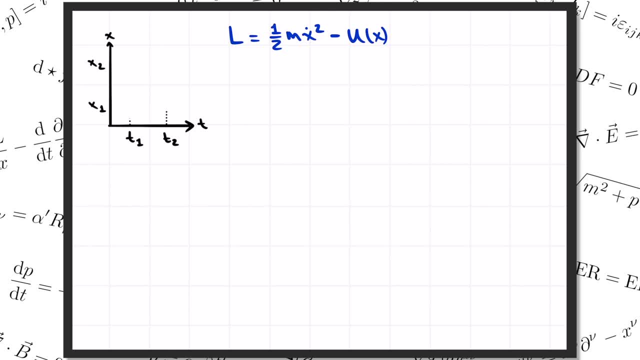 order, the value of the function does not change at all. This is the defining property of an extremal point. The same idea goes for our action and the critical path x of t. If we successfully find the trajectory that minimizes the action, then for any nearby. 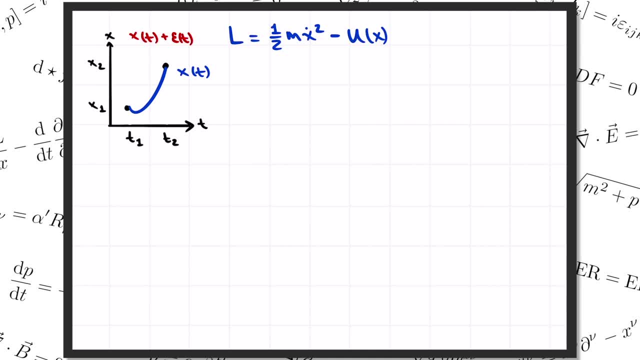 path x of t plus epsilon of t, the value of s should be unchanged, Where this epsilon of t is a tiny variation of our solution that introduces little wiggles along the trajectory. So let's expand our Lagrangian in powers of epsilon. 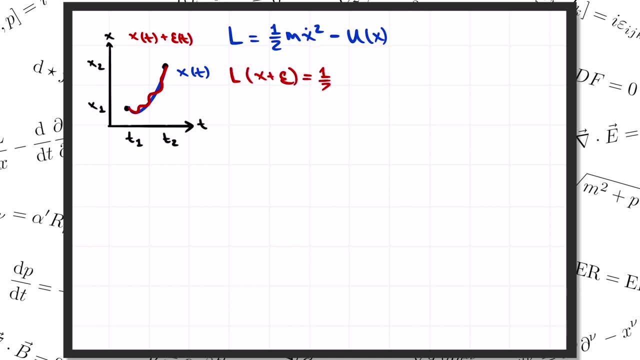 We have L of x plus epsilon. by definition is one half m times x dot plus epsilon dot squared, Minus u of x plus epsilon. If we expand the first term we've got x dot squared plus two x dot, epsilon dot plus epsilon dot squared. 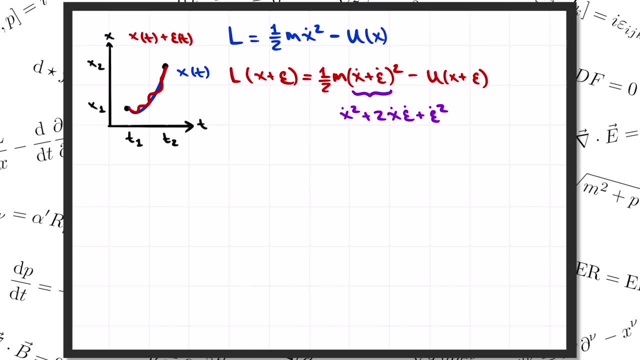 But remember, we're only working to leading order in epsilon here, So we don't care about things with more than one power of epsilon. In the second term we apply our Taylor series again. We have u of x plus epsilon equals u of x plus u, prime of x times epsilon. 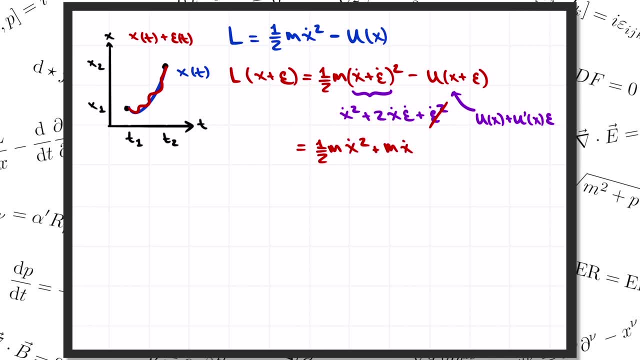 So we get one half m x dot squared. Therefore, u is less than or equal to 1.. And since u was less than or equal to number V, a flashy variation goes out. The change in the Lagrangian method is: miser deceased employers. 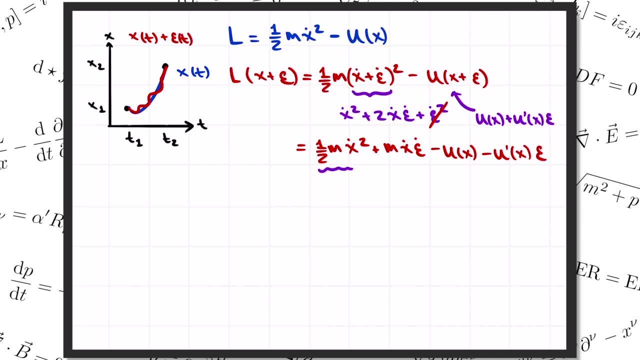 So we've got u prime of x square plus m, x, dot, epsilon, dot minus u, minus u, prime times epsilon. Now notice that these two terms are the original Lagrangian. So if we subtract that to the other side, we've learned that the change in the Lagrangian 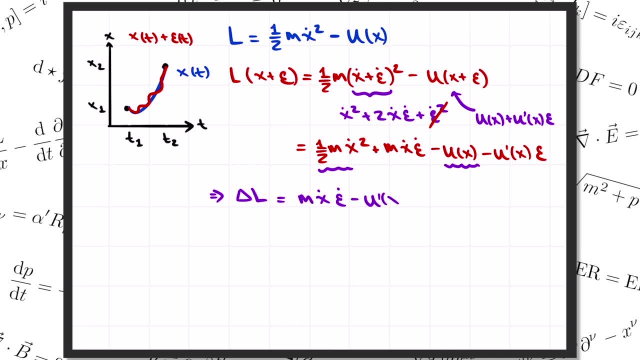 is m, x, dot. epsilon, dot. minus u. prime of x times epsilon. The change in the action is therefore the integral of that And that's what's supposed to vanish. av, mx, dot. epsilon, dot, v, v. We want this to equal zero for any little deformation. epsilon of t. 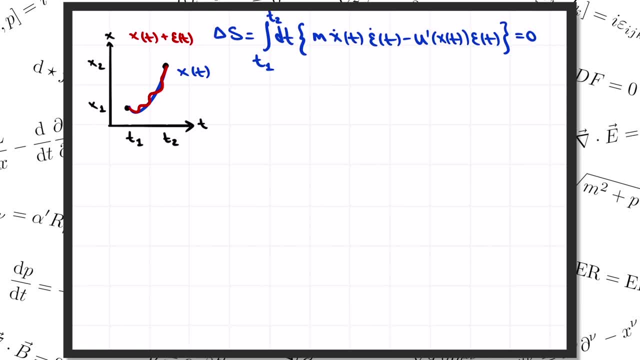 So how are we going to make that happen? Well, it would be nice if we could pull out a common factor of epsilon from the integrand, But in that first term it's epsilon dot that's showing up. So it might help to apply integration by parts to that first term. 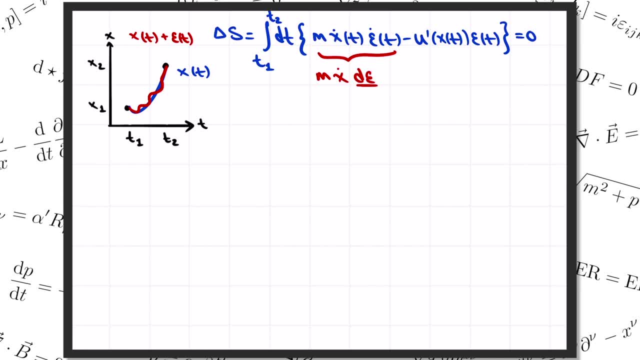 That means that we can rewrite m x dot times d epsilon by dt as d by dt of the whole thing: m x dot epsilon minus m x double dot times epsilon. That's just an identity that follows if you expand out the right hand side by applying 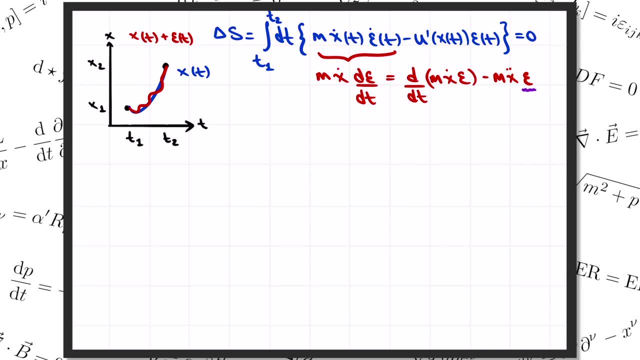 the product rule. Well, now, this second term has an epsilon in it, which is what we wanted to pull out. What happens with this total derivative in the first term? Well, the integral of a total derivative is pretty simple. We're just going to get the difference of the function evaluated on the two boundary. 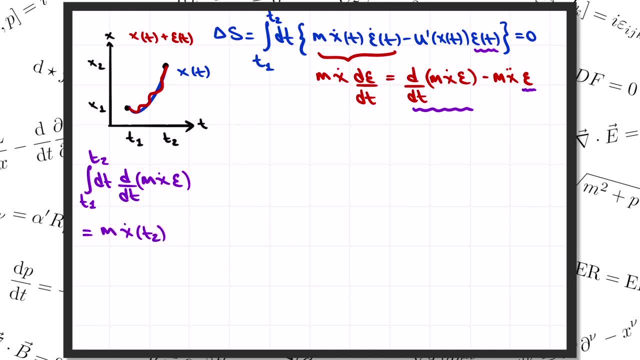 points. That's m times x dot at t2 times epsilon at t2, minus the same thing evaluated at t1.. Remember that we're considering all the paths here that go from the starting point to the end point, both of which are fixed. 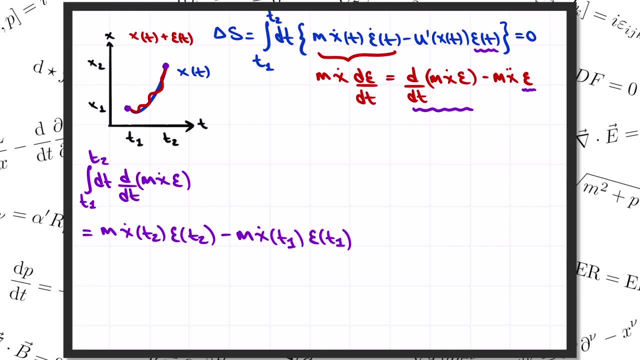 Our deformation is a tiny variation of any such a path, but we don't want it to change the boundary conditions. So, in other words, we're only going to allow epsilon at t2.. That means that epsilon at t2 should be 0 and epsilon at t1 should be equal to 0.. 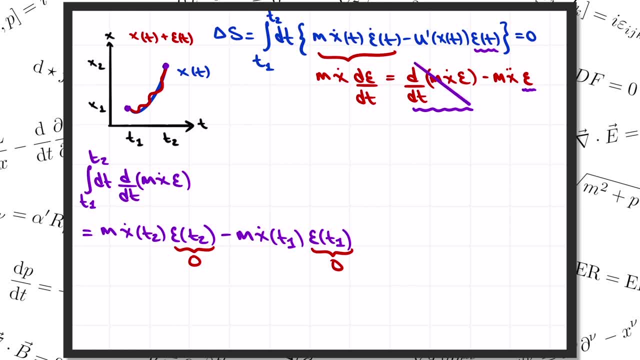 Then the contribution to the action from this total derivative term is just 0.. Therefore, the change in the action is just the integral of minus m, x, double dot, minus u, prime of x, all that times epsilon, That's what we want- to equal 0.. 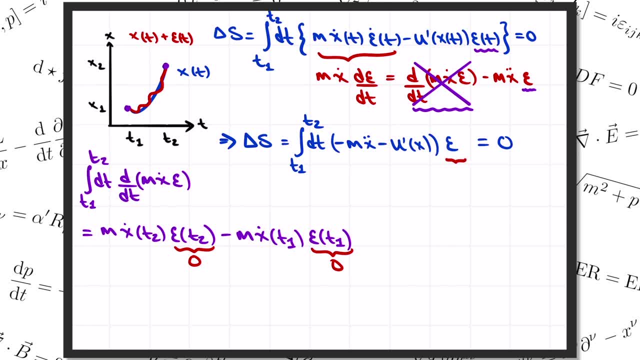 And now we're done. Since this thing is supposed to vanish for any epsilon, This factor in parenthesis has got to be 0.. Therefore we conclude that in order to minimize the action s, the trajectory x has got to satisfy m x. double dot equals minus u prime of x. 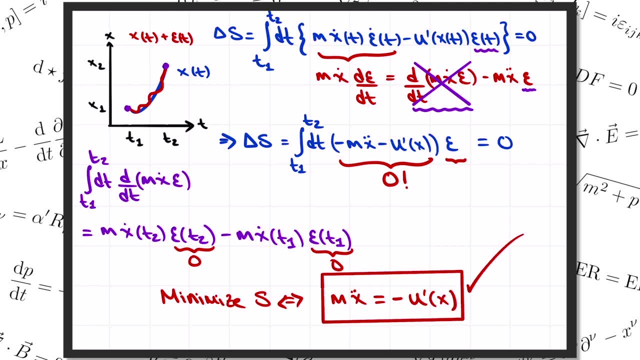 Which is exactly the equation of motion we found earlier from Newton's law. So that proves our claim. Of all the paths that the particle could follow to get from point 1 to point 2, the one that it actually chooses is the path from point 1 to point 2.. 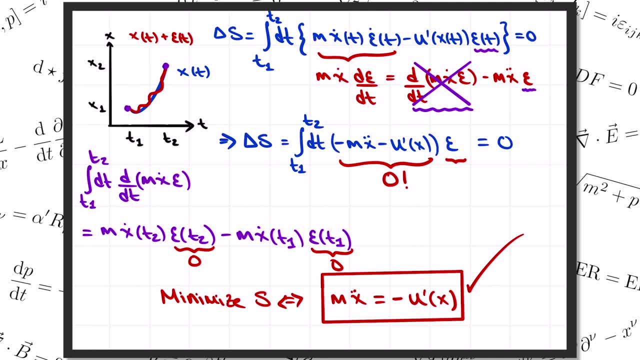 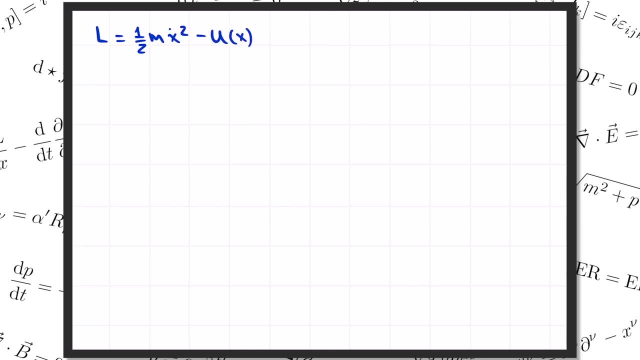 It's the path for which the action s is minimized. This principle of least action is an extremely powerful way of looking at physics, Although if this is your first time encountering it, I imagine you might think it looks a little bit more complicated than. F equals m a. 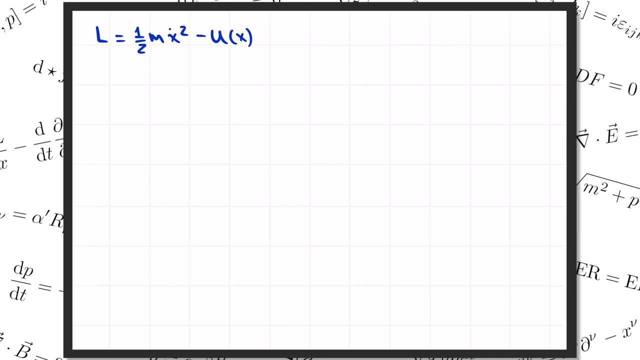 But actually it's very often the most straightforward way to write down the equations of motion for a system. I did things pretty systematically just now, But actually there's a faster way to get to the equations of motion once you know the deal. We're essentially just taking the direction of motion. 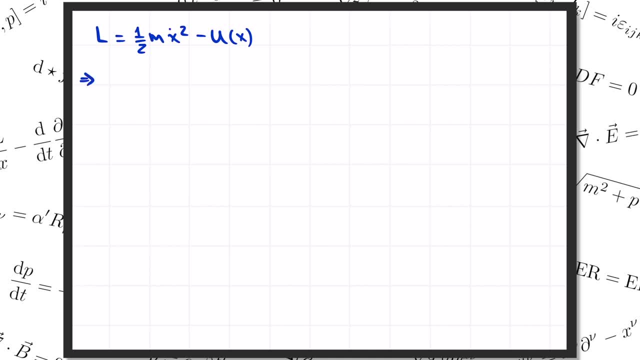 We're essentially just taking the direction of motion, But actually there's a faster way to get to the equations of motion, Because we're literally just taking the direction of motion, But actually there's a faster way to get to the equations of motion. 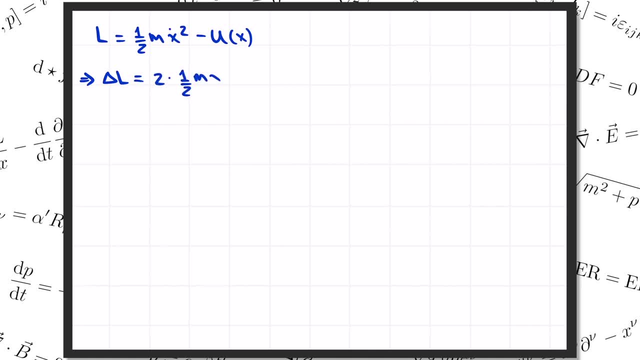 To find the change in L, we just get 2 times one half mx dot times the change in x dot, which is epsilon dot Minus u prime of x times the change in x, which is epsilon. Now we integrate that to get the change in the action. 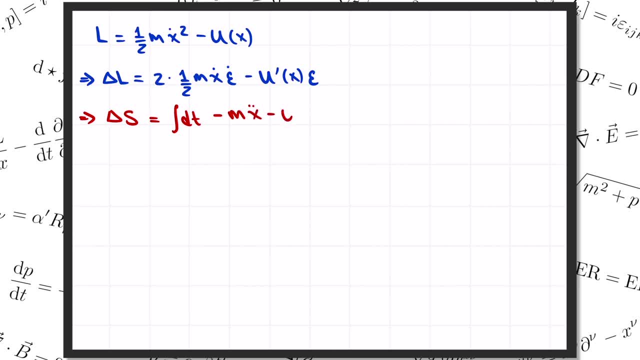 And we integrate by parts to move the derivative off the epsilon and on to the x double dot And just like that we've got the equation of motion. So bit of practice. you'll be able to do all that in your head and go straight from the. 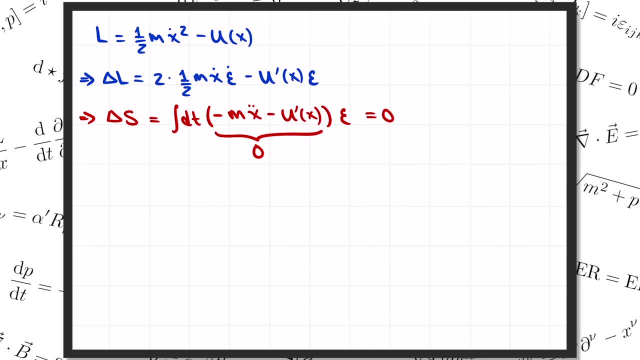 Lagrangian to writing down the equation of motion. Of course all this generalizes to systems with multiple particles and multiple dimensions. You can even find the general minimization condition once and for all by taking the variation of the action for a general Lagrangian L, which is some function of all the x's and 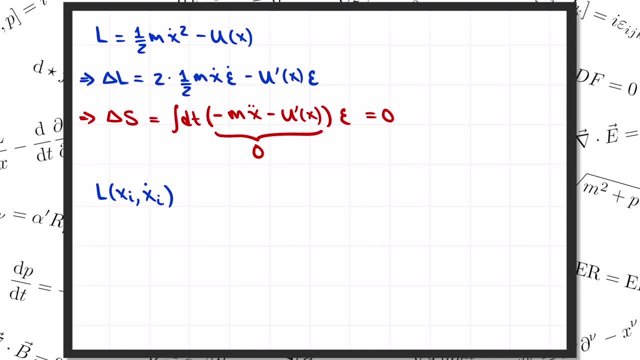 all the x dots for the coordinates of any number of particles. I show you how this works in the notes that I wrote, to go along with the video which you can get for free at the link I'll put down in the description. The result is that the action will be minimized if the time derivative of dl by dx dot is. 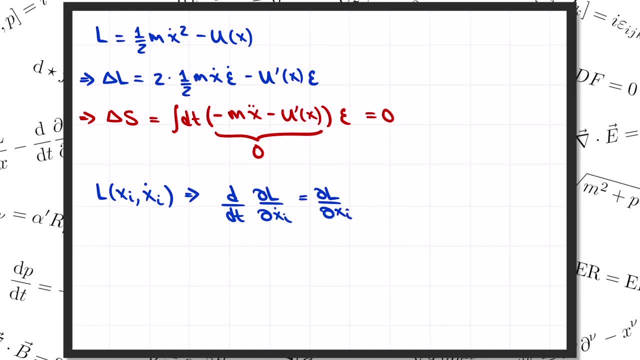 equal to the derivative of L with respect to x for each coordinate. These are called the Euler-Lagrange equations, and if you want to see an example of how they're applied, check out the earlier video I made, which I'll link up in the corner. 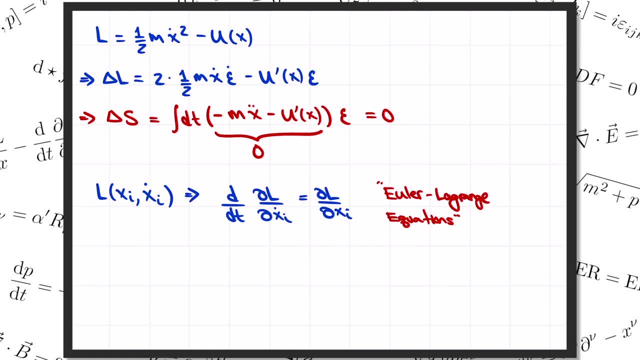 These squiggly derivatives here are partial derivatives. They behave just like regular old derivatives. it just means that we're going to pretend everything else in the Lagrangian is a constant when we take the derivative with respect to x or with respect to x dot. 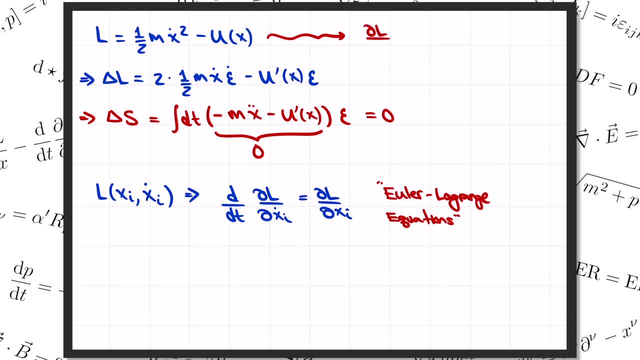 So for example, for our Lagrangian here, the derivative of L with respect to x is minus u prime of x. The derivative with respect to x dot is m times x dot. And then when I take d by dt of that I get m x. double dot equals minus u prime of x. 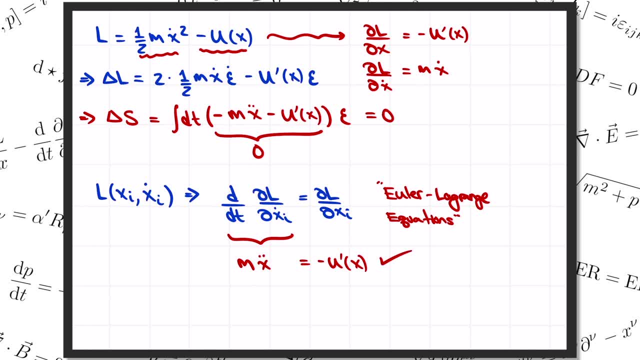 So this Euler-Lagrange equation indeed reproduces our earlier equation of motion, just like we found by explicitly taking the variation of the action and setting it equal to zero. As a matter of fact, most of the time, physicists compute the equations of motion like I showed. 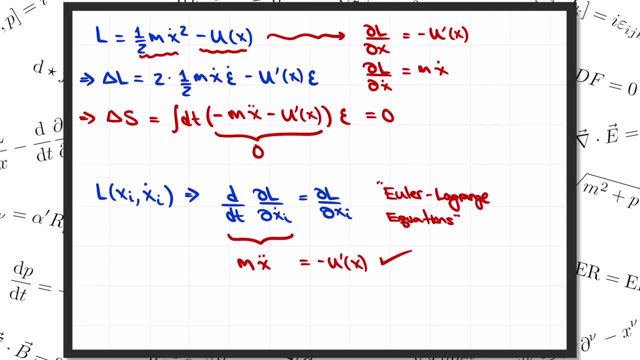 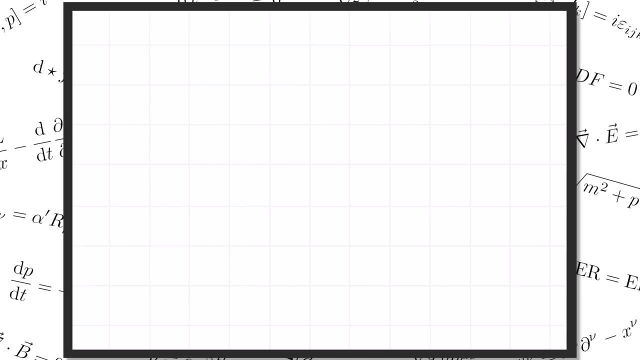 you by taking the explicit variation of the action, rather than having to remember the form of these complicated Euler-Lagrange equations. Now, all this might seem a little bit mysterious, or even miraculous, if this is your first time learning about the principle of motion. 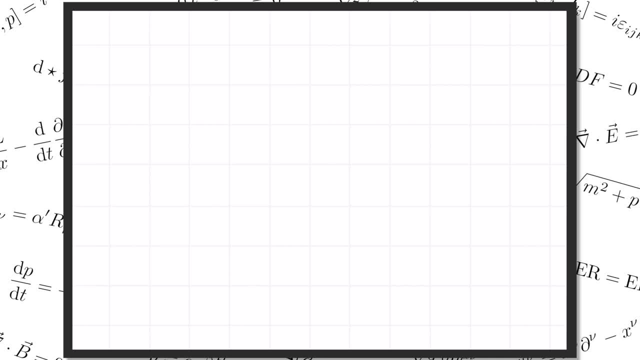 Where is all this coming from? Well, the last thing I want to do is briefly describe how the principle of least action arises from the classical limit of a more precise quantum mechanical treatment of motion, Although if you haven't learned quantum mechanics before, I suppose this will be even more mysterious. 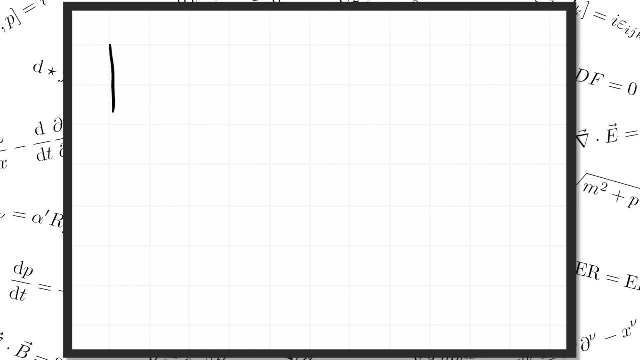 But hopefully you'll be inspired to go off and keep learning more In quantum mechanics. all we can say is that the particle has a certain probability of traveling from its initial point to its final point. The rules of quantum mechanics tell us how to compute the transition amplitude, which 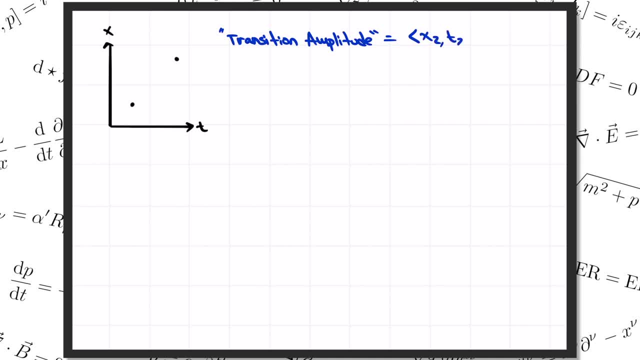 we usually denote like this the amplitude to go from point 1, at time t1, to point 2 at time t2.. The probability is then given by the square of the amplitude. The famous physicist Richard Feynman showed in his PhD thesis that this amplitude is. 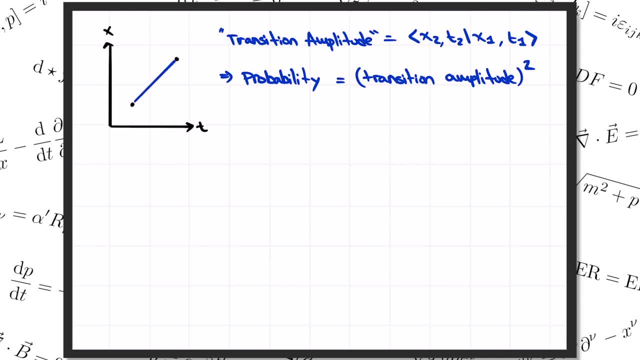 related to the action as follows: We consider all the possibilities of the transition amplitude to be equal to zero. We then assign all the possible paths from the starting point to the end point. Assign a number to each path given by e to the i times s the action divided by h-bar. 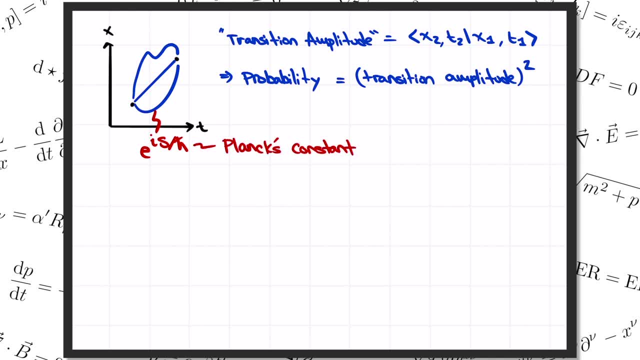 where h-bar is Planck's constant. it's a number that characterizes the scale of quantum mechanical effects. Then the particle takes all the possible paths from point 1 to point 2. And if we add up these weights for each path, Feynman tells us, we get the transition amplitude. 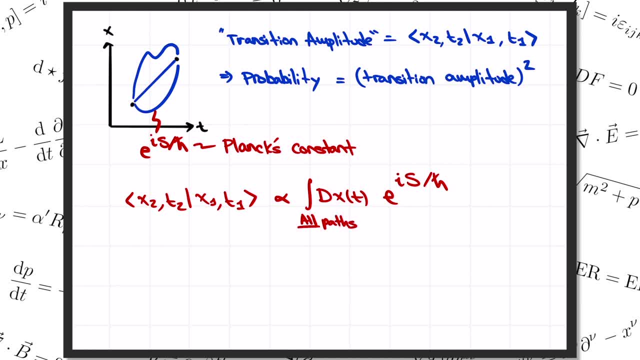 The integral here stands for the sum over all the paths from the starting point to the end point. It's therefore called a path integral. It's more complicated than the ordinary integrals you're familiar with because we're not summing over a regular variable here. 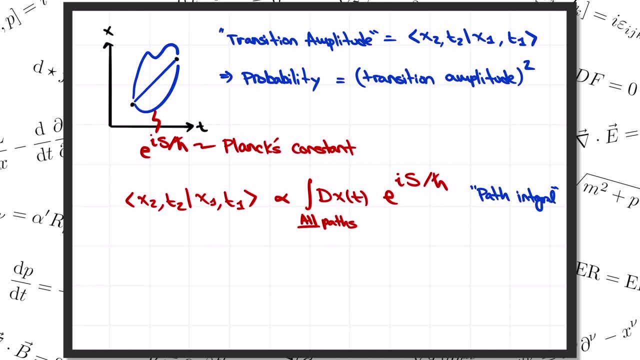 We're summing over functions x, And yes, you're right, This is totally nuts. We're saying that the particle takes every path from point 1 to point 2. And then we add them all up. It's crazy, But that's quantum mechanics for you. 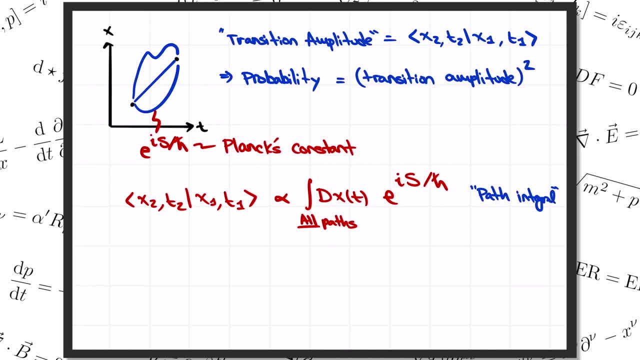 Now, what is this? What is this? What does this have to do with the principle of least action? These weights, e to the i s over h-bar, those are phases, meaning that they're complex numbers of magnitude 1.. In other words, they're like arrows pointing on a circle of radius 1.. 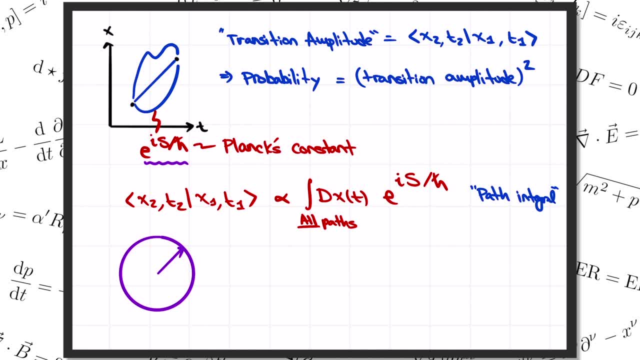 When you add up all the weights for all the paths that the particle can take, these arrows mostly point along in random directions around the circle and they add up to 0.. The exception is for the paths near the one that minimizes the action. 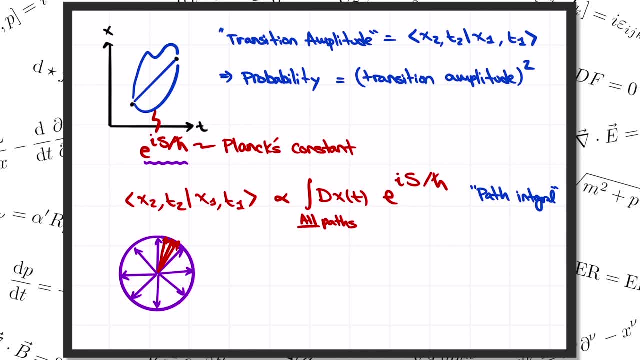 Ahちょ ở tître k café. Because, remember, for those paths the action isn't nearly constant as, by definition, the action doesn't change to leading order around the minimum. Then these contributions near the classical path almost all have the same weight. 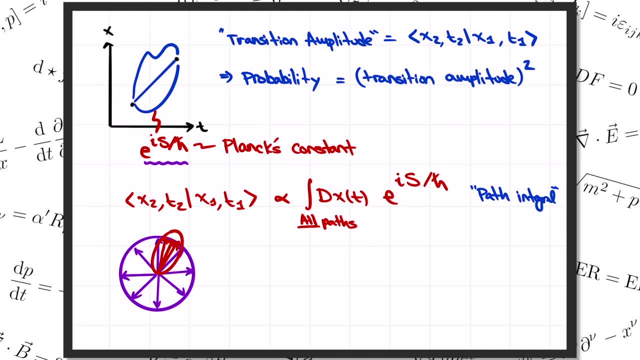 And those arrows add constructively instead of canceling out. The result is that the path integral IS dominated by the trajectory that minimizes the action Which, as we've seen, yields the classical solution. So the amplitude IS dedicated to the opposite trojan. 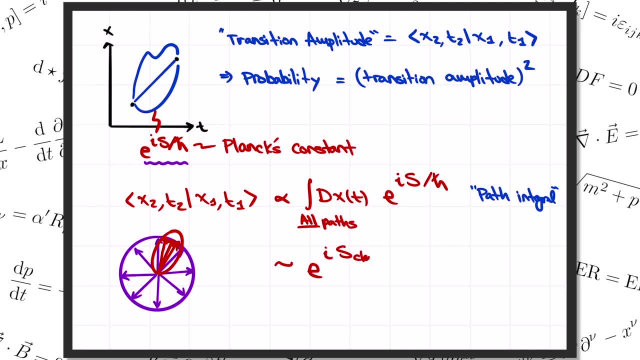 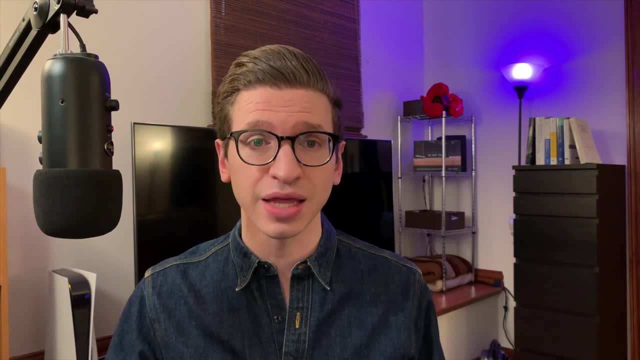 Okay, dominated by e to the i times the classical action divided by h-bar. This is how the principle of least action emerges from quantum mechanics, Of course. now it's only fair that you should ask why the heck this path? integral computes the probability, like I claimed, but that'll have to wait for a video of its own. 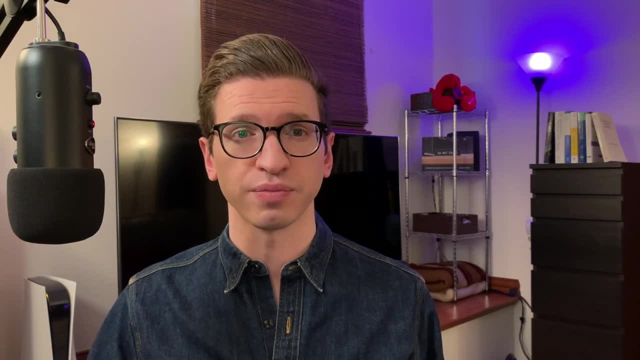 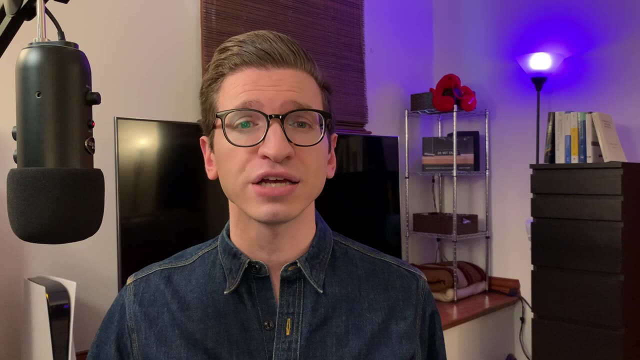 I focus here on the simplest action for a non-relativistic particle, But the applications of the principle of least action go way beyond that. In some upcoming videos I'll show you the action principle for a free particle in special relativity and in general relativity. Einstein's theory of gravity.